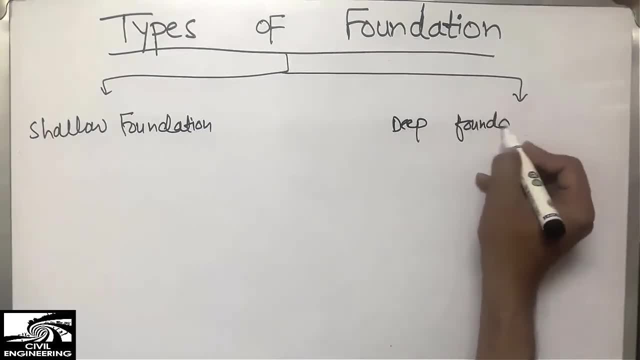 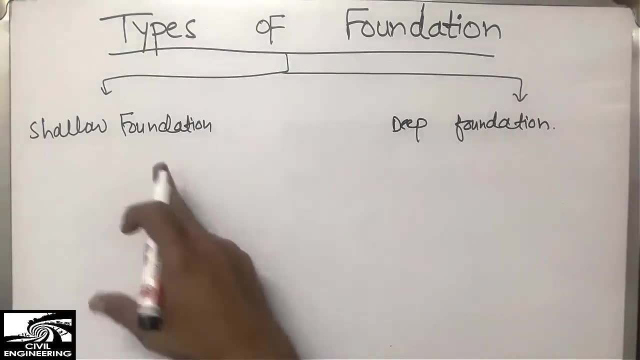 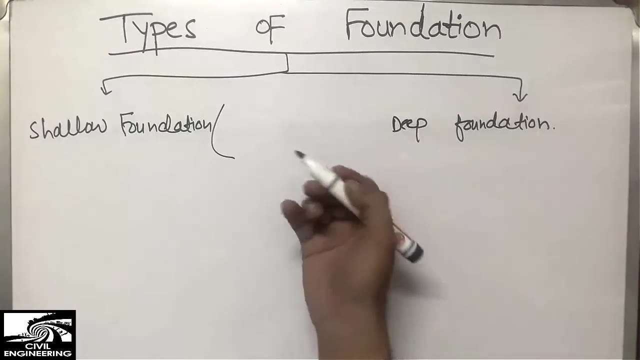 These are the two main types of foundation. Deep foundation- right So the shell foundation is used mainly for the residential. These are the two main types of the foundation. Deep foundation- right So the shell foundation- is used mainly for the residential buildings, where there is not too much load on the side and the side being pissed is low, we can say, and there is not too much load coming on these and the side. 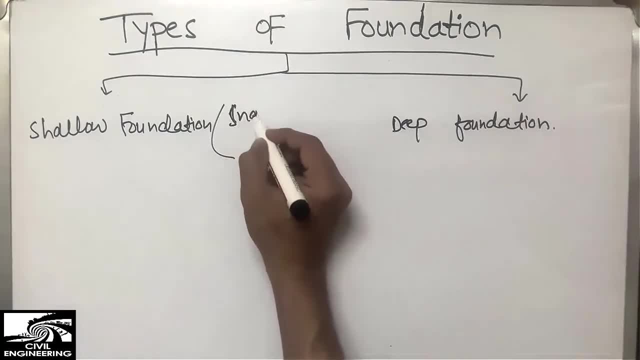 So we provide the shell foundation, So it's provided mainly for the. we can say it's mainly provided for the small load coming on the side right Or small loads of superstructure. we can say We provide the shell foundation, But deep foundation are provided when there is a huge load coming on the side. 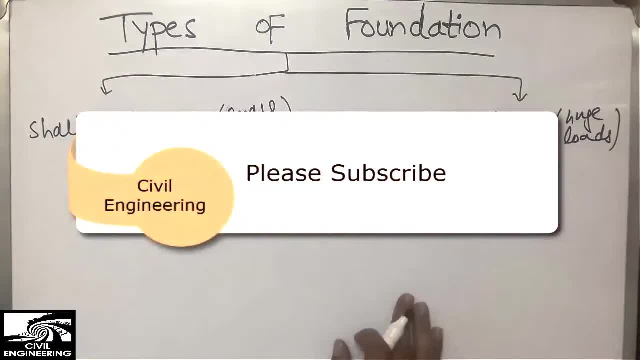 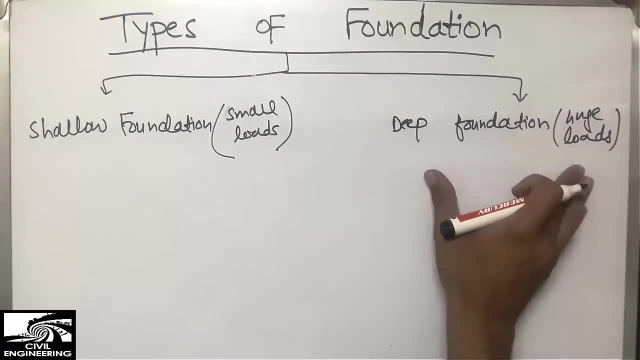 So we provide the deep foundation right. It's the main difference between these two. So when to provide this one and when to provide this one, It's mainly for the huge load coming on the foundation. It's when the small load is coming on the building, mainly the residential buildings. 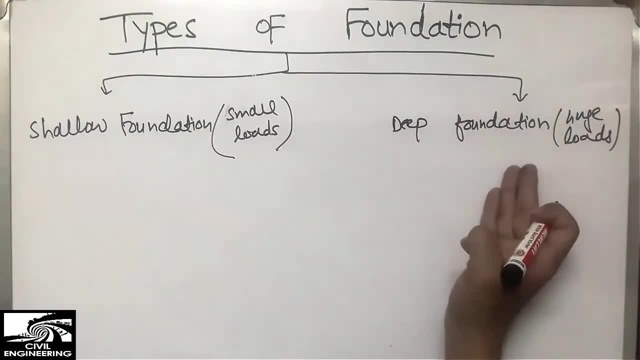 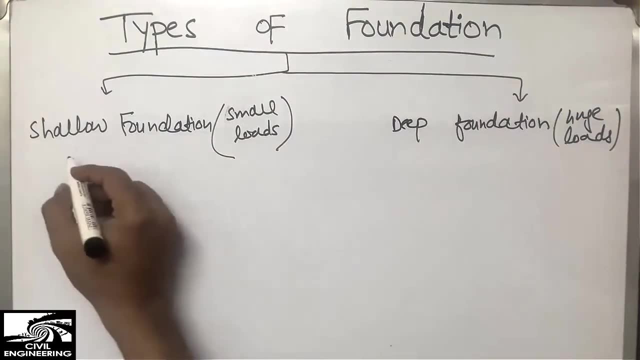 It includes, while this stuff include the bridges, structures, we provide the deep foundation right. And the other thing is the Tarzah. he states that when the Tarzah, which is the father of soil mechanics, he states that the 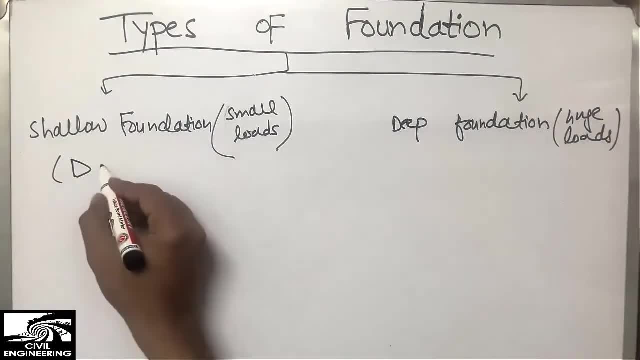 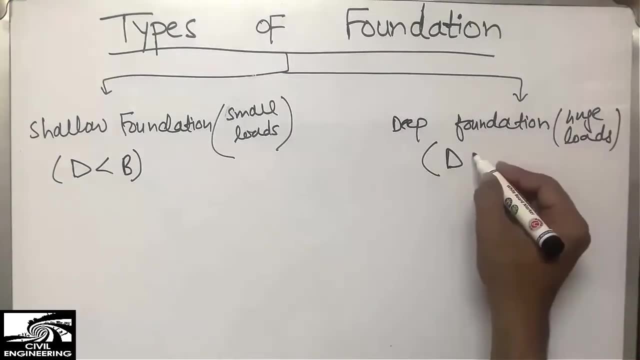 when the depth of the soil, when depth of the foundation is less than the width of the foundation, we call it shallow foundation, and when the depth of the foundation is greater than the width of the foundation, we call it deep foundation. this is the other classification of how to 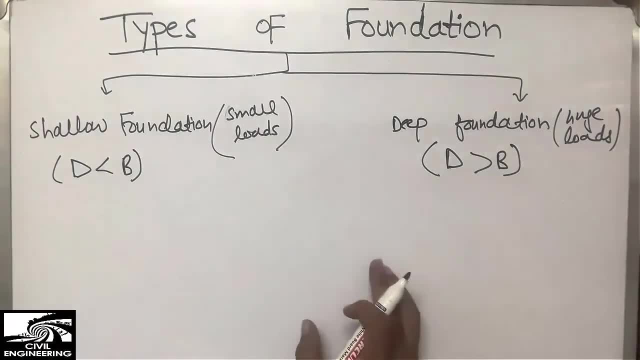 classify the shallow foundation as well as the deep foundation. so now, uh the uh we are. we are going to discuss now the uh types included in the shallow as well as in the deep foundation. right, because there is no such a foundation provided everywhere, but there are the types, or some types. 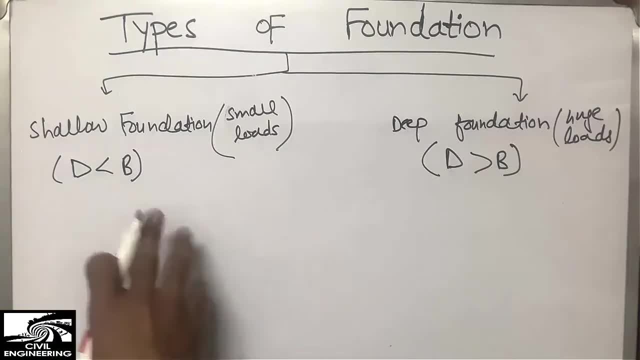 which are included here. now i'm going to discuss these types, and these types are used in a different condition, according to the load, according to the foundation condition. so the shallow foundation is further classified into main four types. right, the first one is spread footing or spread foundation. 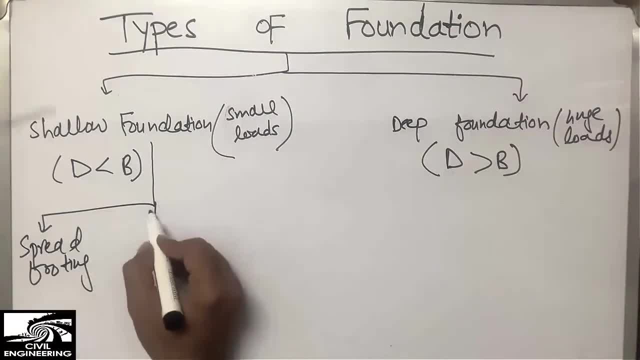 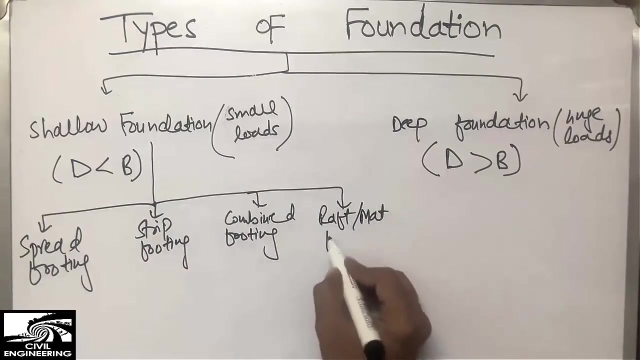 the second one is the straight footing, or strip foundation, and it's also called wall footing right. and the third one is combined footing- combined footing. and the fourth one is raft, or made footing right after made footing. these four are used according to different conditions. right, no one. no one more. engineer. 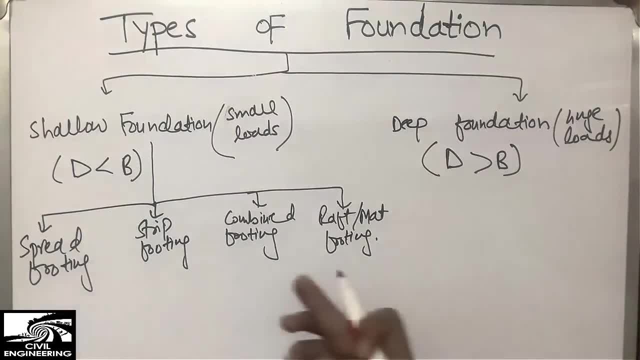 can use uh in one, throughout the throughout his project. uh, only one type of foundation he can. he might change the foundation types according to the condition of the load, according to the condition of the soil strata. right, so split footing is mainly used. i'm going to discuss one by one in detail. right, the split foundation is mainly used for. 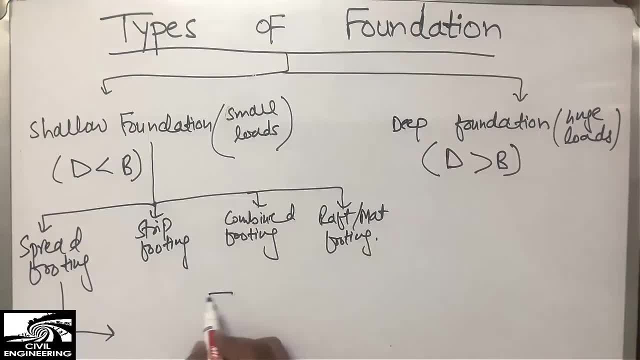 the column for a single column like: this is the column, this is the footing we provide, and this is the column and the footing for the one column. this is the column and the footing provided to support the one column we call is the spread footing right? this, this is the column we provide: the reinforcement. 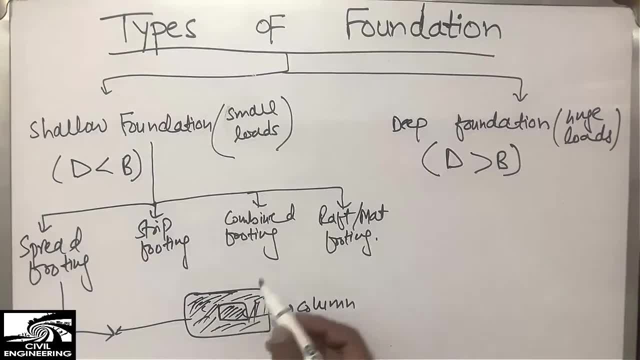 in both directional and that to support this column and the column load is coming uh to this. now the the column load is coming and this footing will support this column load and it's uh being called a spread footing, right, it's also sometimes called isolated column footing. 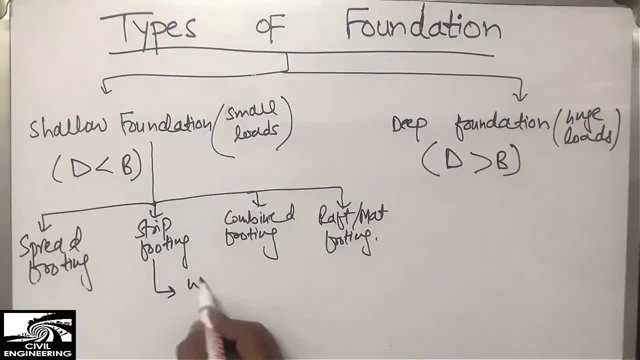 now coming to the second types. it's called strip footing, are also called wall footing, or strip footing are also called wall footing. it's provided mainly throughout the wall, like this is the wall and drawing it here. this is the wall- right wall- while the foundation, the footing, placed below the 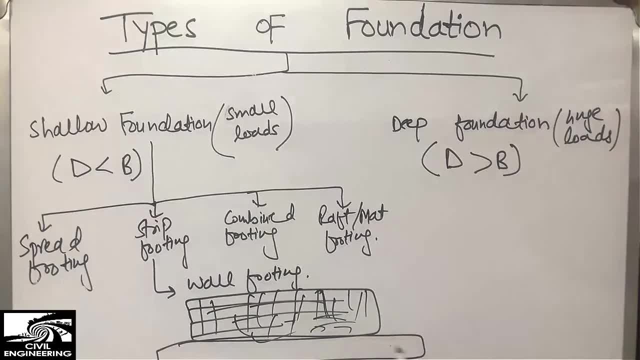 wall. we call it like this: is the wall footing. we provide this, the footing, uh, for the wall. this is the wall and we provide the footing for the wall. so it's called is wall footing or strip footing. it's only it's like a strip, it's. 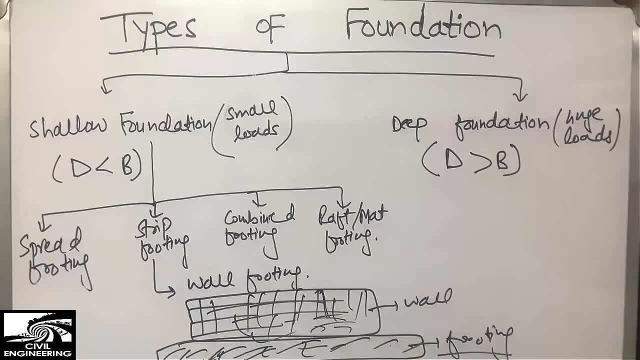 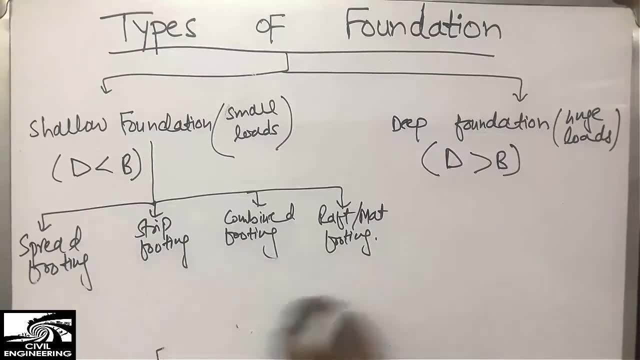 name shows that it's like a strip provided underneath of the wall. so we call: is the strip footing right? this was the second type of the shell foundation. now i'm going to discuss the third type of phone footing shell foundation. it's called combined footing, compound footing. 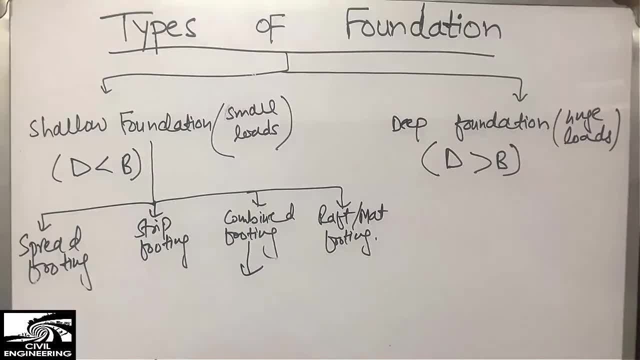 is used when the uh compound footing is used mainly when. but there is, or like, for example, the one column is here, one column is here, so we are not going to place the. these are the columns too. we're not going to place the split footing, like for this one, for this one separately, but we 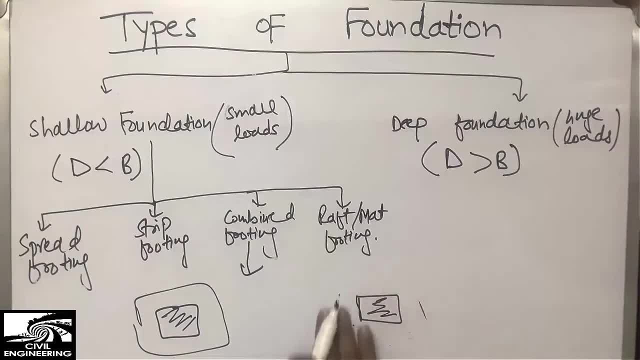 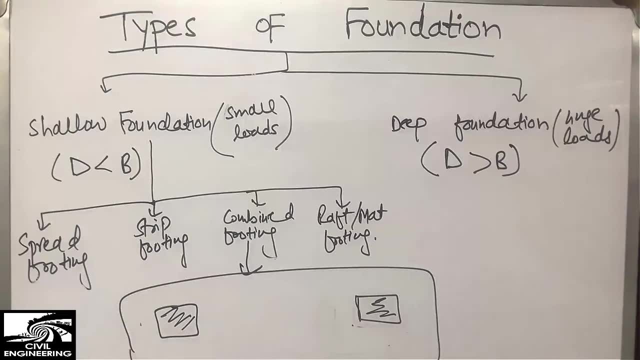 place the foundation, uh for the combined foundation for both this column so we call is combined footing. like i'm going to place such type of footing and to support this two column and the load is coming and this uh from the two columns and it will undergoing to this type of uh footing and we call this footing is. 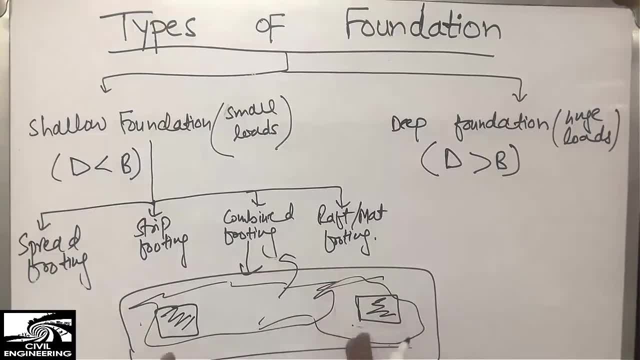 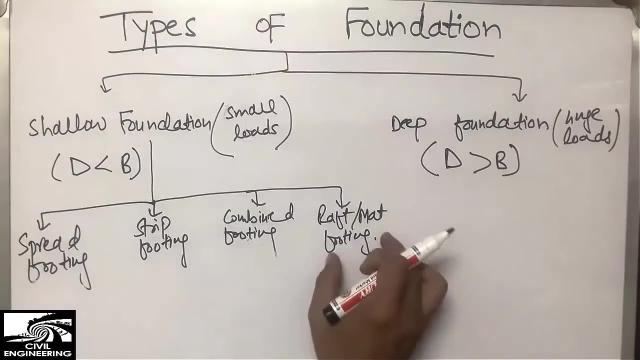 the combined footing right because it's now combined the two columns- is being supported to this type of foundation. it's called now is combined footing. so this was the third type of shell foundation. now coming to the raft, or made foundation, is the third type and it's mainly this type foundation is. 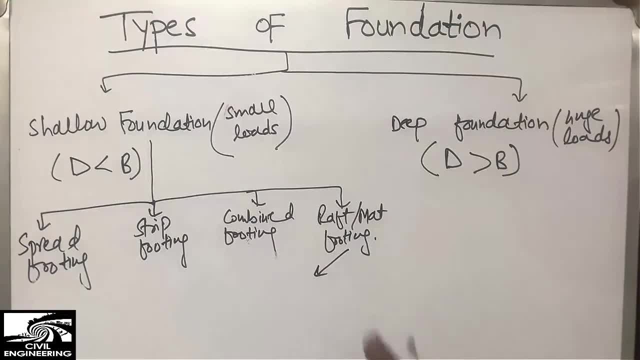 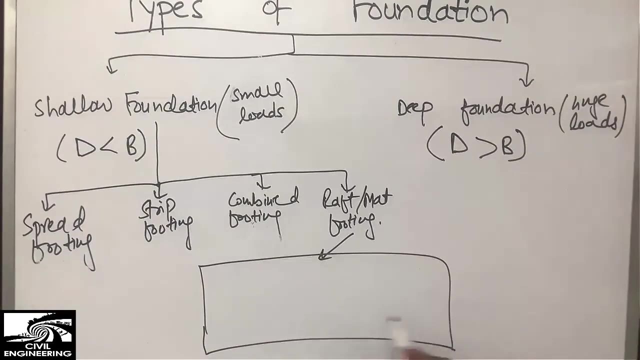 mainly provided to support a huge load coming on this side straight right, because, uh, this type of footing is mainly like in this way, in this right, uh, in which the two columns are: these are the different columns. sorry, there's different columns, provided circular or maybe rectangular, and the whole area may be circular or rectangular. 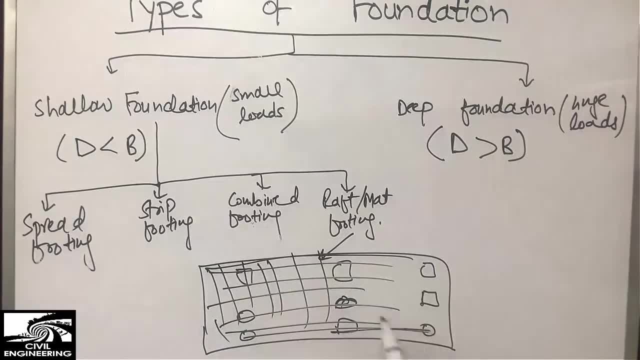 sorry it may be, square or rectangular, is throughout the depth, is wholly reinforced with the steel bars and this whole area is now reinforced and it's the concrete is placed in this area and the columns are placed also in this area, so it's a huge type of sleeve we can see. 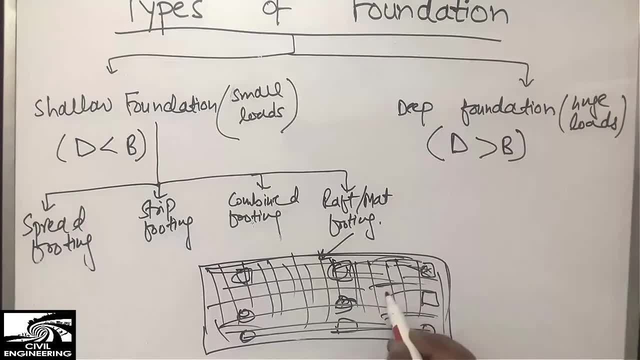 the base sleeve. sometimes it's also called base sleeve because it's a very huge, concrete, solid sleeve and it can support more demand as compared to these three type of footing. so we call is raft or made footing, and it's providing mainly to support the huge load coming on the foundation and and which will first place the 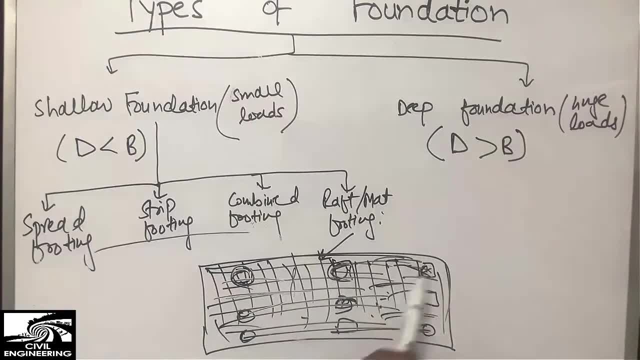 reinforcement and then we place the uh column reinforcement and then place the concrete so it uh, very huge uh type of slab is created below support the upper load, so this type of foundation will provide scarlet. they made a rough footing and it's mainly for the huge load right. 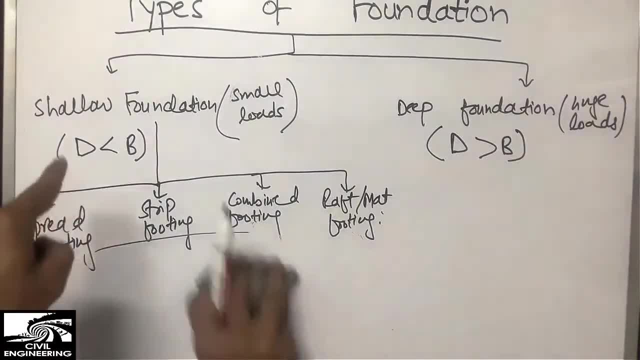 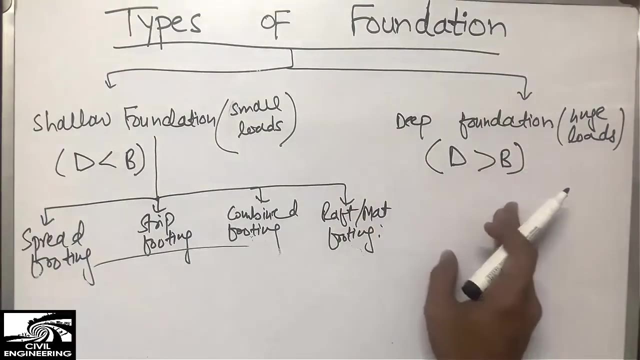 it should be remembered that it can support a huge load. but it's also included in the shell foundation because, uh, it's uh, because it's not provided a very deep uh under the uh in the earth surface, right? so coming to the deep foundation, which is the main type of the foundation and deep foundation, 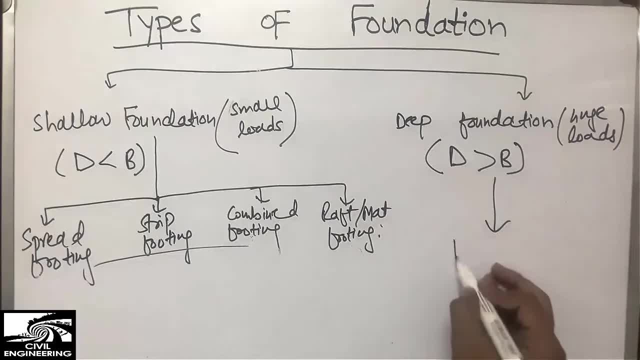 uh, we have one main type foundation is the pile foundation, right pile foundation. uh, further in pile foundation we have another. we have three other types in varying piles, and the second one is friction piles, inbending pile, friction piles and the third one is friction friction, come bearing piles. 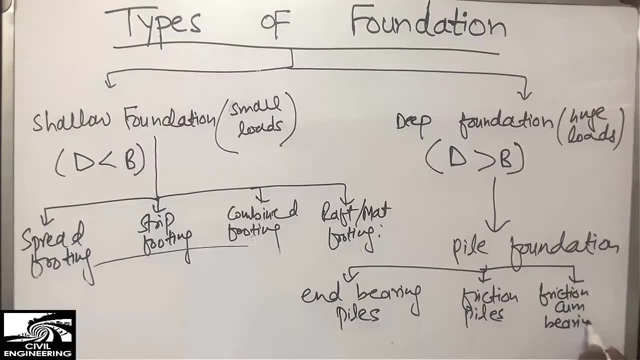 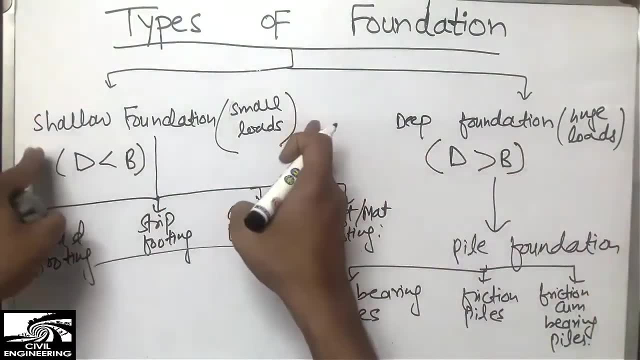 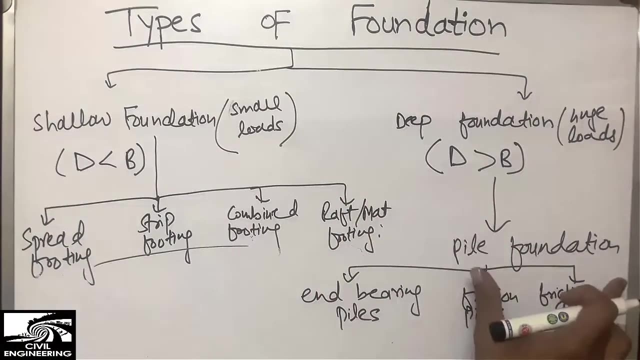 right. so from this coming from shell foundation to deep foundation, this can support a small load, while this can support a heavy load, while this is going under deep, the uh ground surface, right. so the pile foundation can be realized into three types: inbending piles, friction piles and the third one is friction. 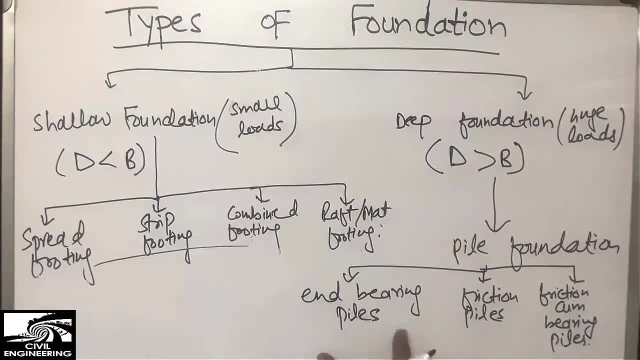 inbending piles, friction piles and friction come bearing piles. inbending piles are used where the strata of the earth surface below the pile is hard. so we provide the inbending piles and in case of the inbending pile, like there's a pile. 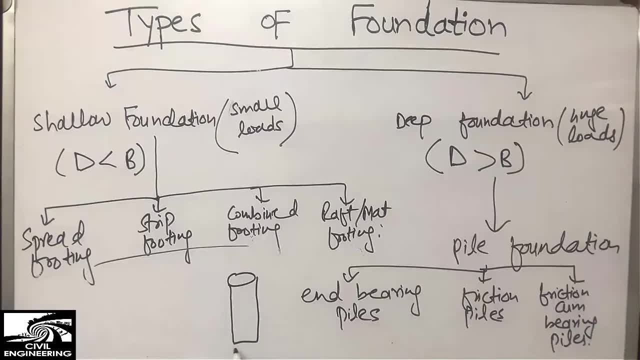 and this is go under the earth surface and the strata provided below the pile is really hard rock strata, so we call it the in pile inbending piles, while when the strata below the- uh, below the pile- is very soft, same dislike, so we call this friction piles, because 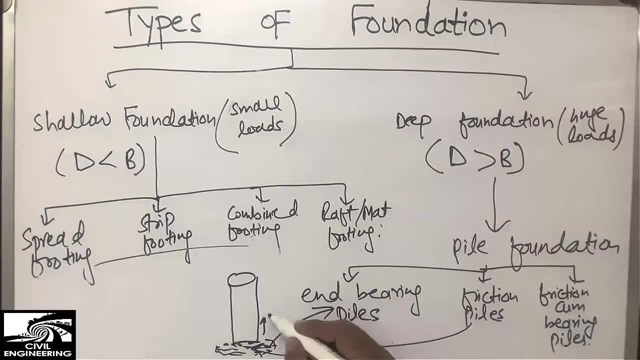 now the resistance in this? in this case, the resistance will be provided by the uh. by the side, uh, way by the side of the piles- and we call it friction piles, right, because the strata are below the pile- will be now the weak. so the only resistance we provided to the skin. 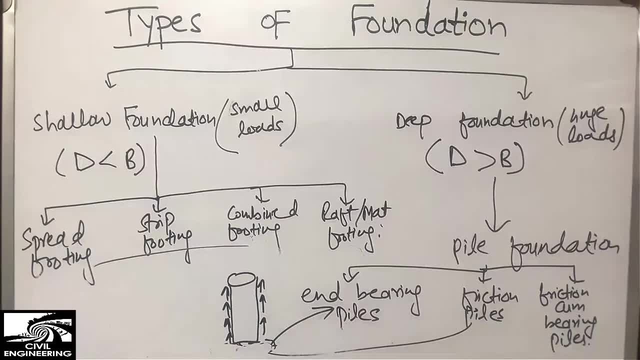 of the pile, in the case of the friction piles right and the friction combining pile. this is the third one. it's provided when the both the strata uh is hard also hard and also the resistance also offered by the uh by the sides of the side. so we call this the 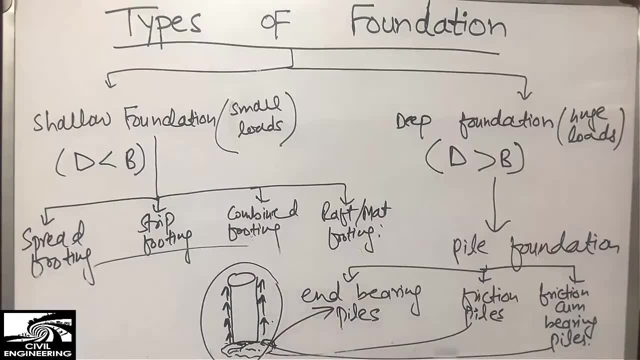 friction, comparing pile right. uh, this was some a little bit. we talk about the pile foundation, uh, also the deep foundation in the shell foundation. so this was today's topic was about the types of formulation and if you any question, please feel free to ask me in the comment box below. 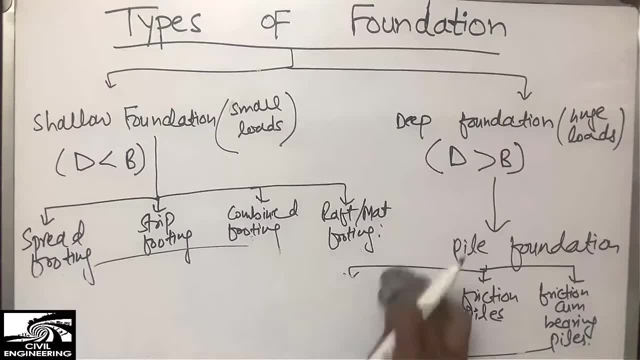 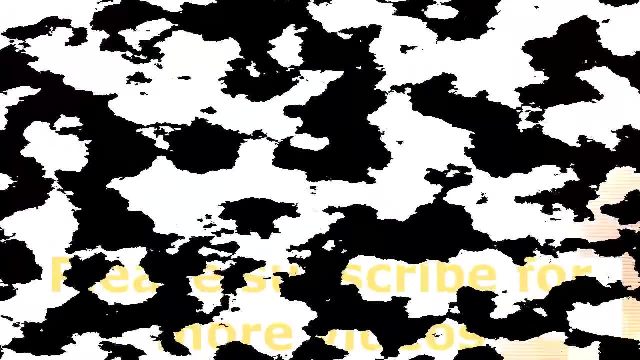 and uh, you can comment. uh, we will respond to you as soon as possible and please don't forget to subscribe our channel for more civil engineering videos. and thank you for watching our video.